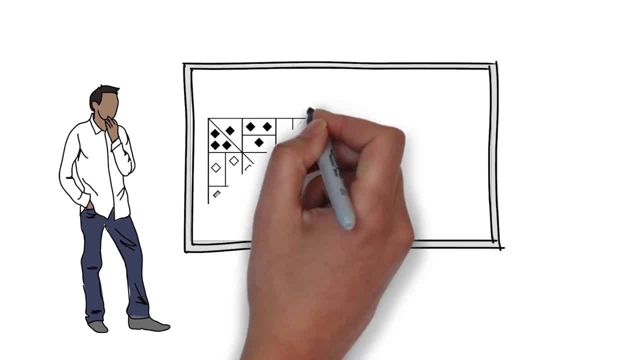 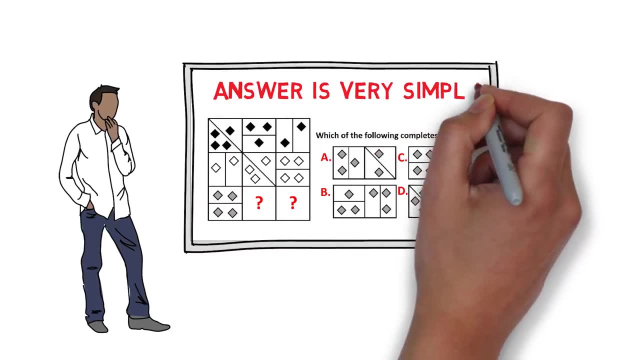 When you see a question like this, you might ask yourself how can it possibly be even more confusing? But the reality is that the answer to the question I'm about to show you is very simple. Let's look in more details. You're presented with the 3x3 matrix. Two of the shapes in the 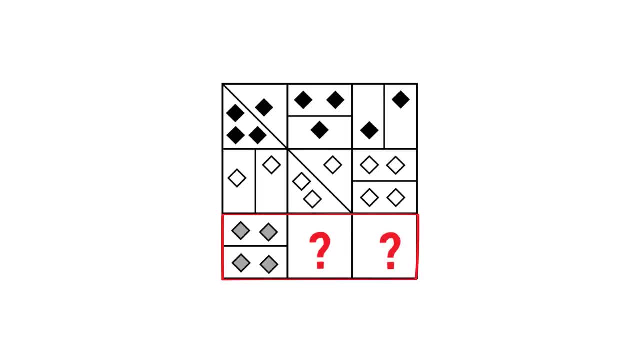 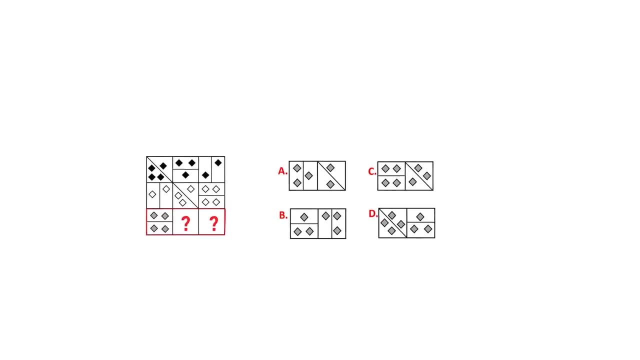 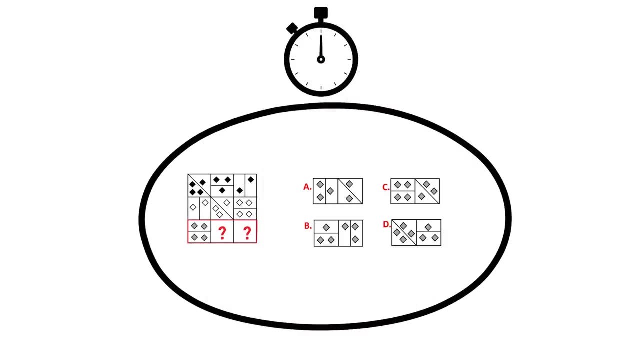 matrix are missing. They are located in the bottom row And you have four possible choices for the answers: Choices A, B, C and D. Take a close look. The solution is not obvious, but it is very simple. Give yourself 10 to 20 seconds, maybe go to 30 seconds by pausing this video to see if you 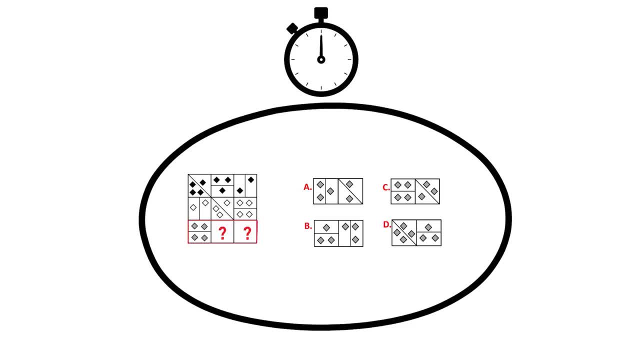 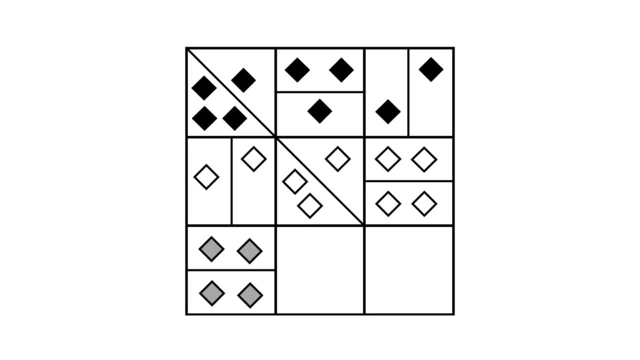 can come up with the answer on your own. Are you ready? Let's continue to see how we can get to the correct solution together. As I mentioned, the answer to this question is very simple. The pattern is represented in each row by decreasing number of diamonds. 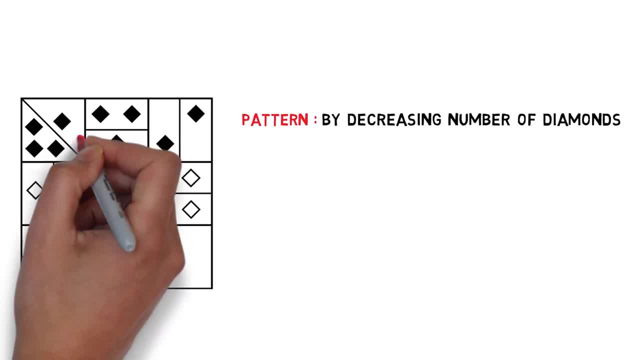 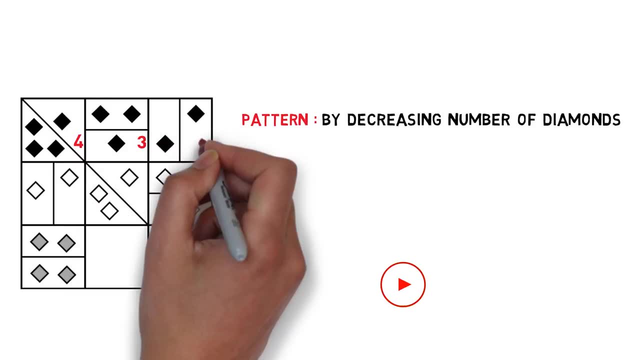 Let's look at the top row. You see that the top left square contains four black diamonds, The middle square in the top row contains only three diamonds, And then the right square in the top row contains only two diamonds. In the second row the pattern reverses and it goes from right. 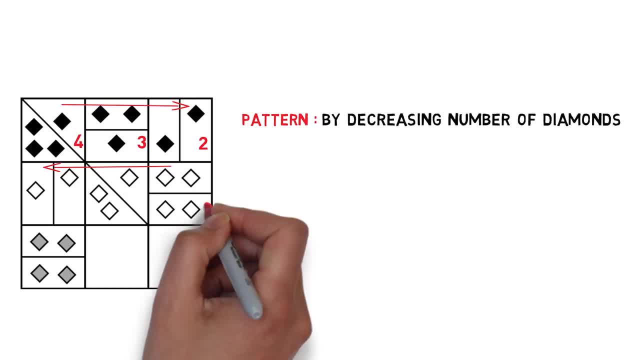 to left And you see the same pattern of the white diamonds. Four goes down to three and then goes down to two. So in the bottom row we need to follow the same pattern. The pattern will be the number of diamonds decreasing from four to two. 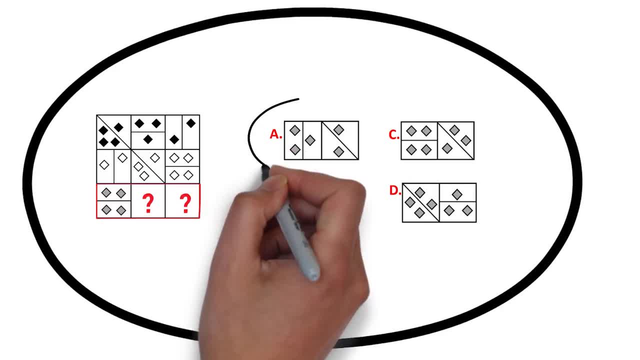 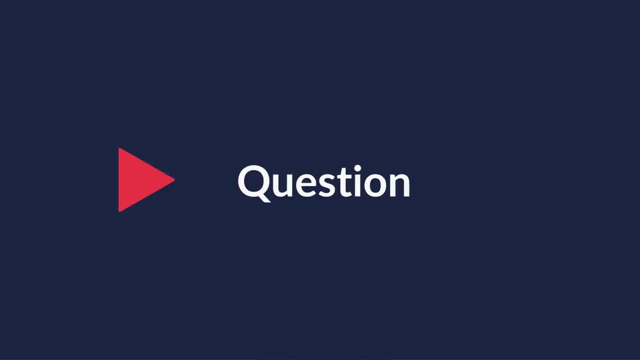 Among the gray diamonds. So the correct answer here is choice A. Hopefully you've nailed this question and now know how to answer similar problems in the test. I'm excited to share with you a cool question which is easy to understand but which doesn't. 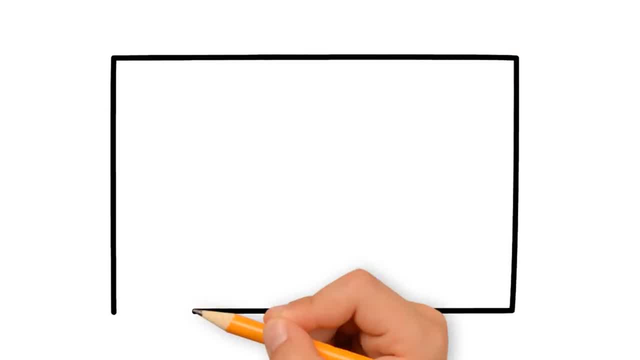 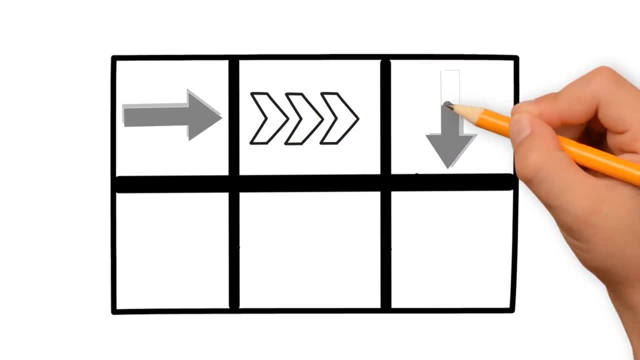 have an obvious answer. You're presented with the 2x3 matrix. This matrix has arrows inside. There are two types of arrows: solid arrows, and then there are arrows that consist of three different shapes. There are two types of arrows: solid arrows, and then there are arrows that consist of three different shapes. 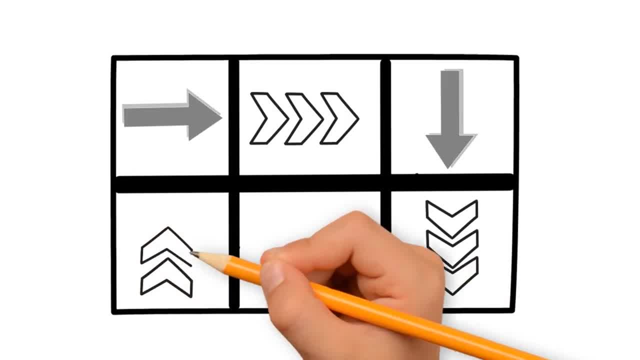 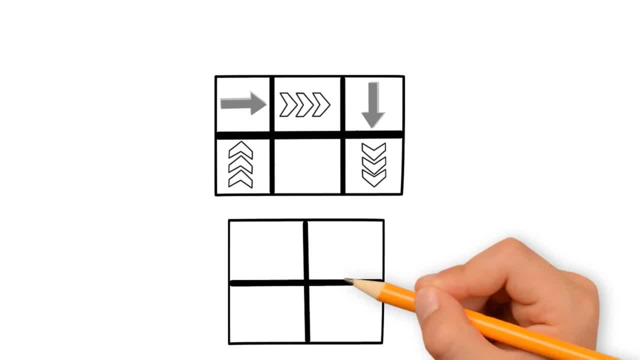 There are six possible spaces in the 2x3 matrix. Five shapes are present and one shape is missing. You're presented with four different choices to identify the missing shape, which is highlighted by the question mark. You have choices A, B, C and D. Give yourself. 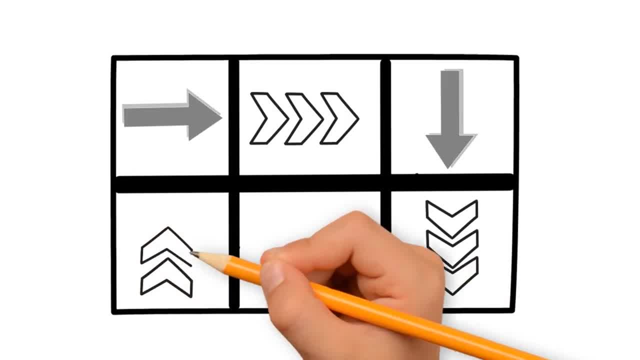 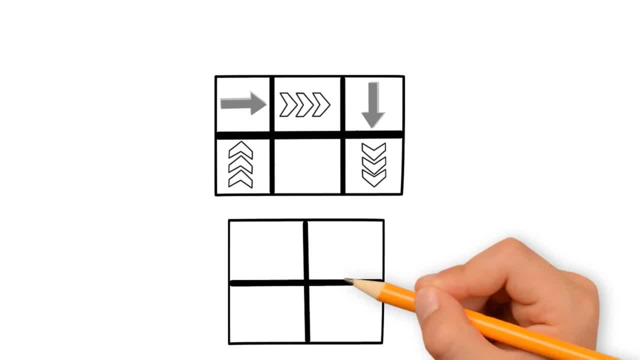 There are six possible spaces in the 2x3 matrix. Five shapes are present and one shape is missing. You're presented with four different choices to identify the missing shape, which is highlighted by the question mark. You have choices A, B, C and D. Give yourself. 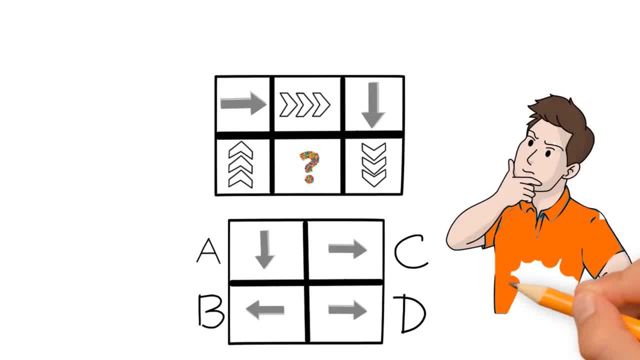 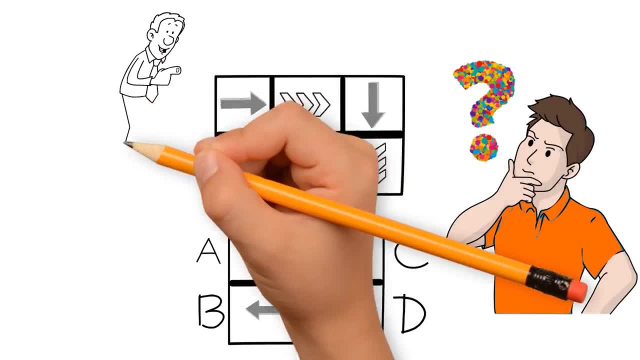 10 to 15 seconds to see if you can identify the right answer. Did you figure out the correct answer? Let's continue to see if we can get to the correct solution together. To solve these types of challenges, you always need to look for patterns. 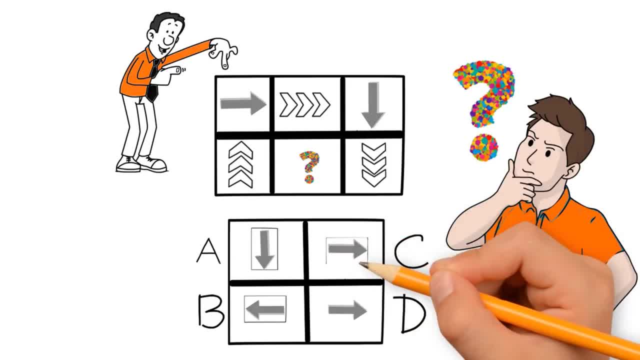 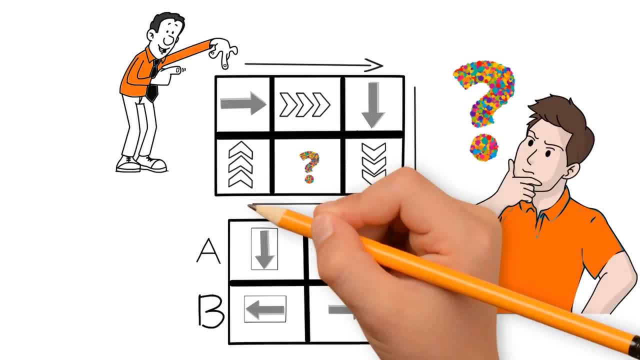 And there are three different patterns present in this sequence. Let's look at the pattern 1.. If we start from the upper left corner and go clockwise, you see that the arrows change alternatively in each subsequent box. Second pattern is that inside the box, solid arrows. 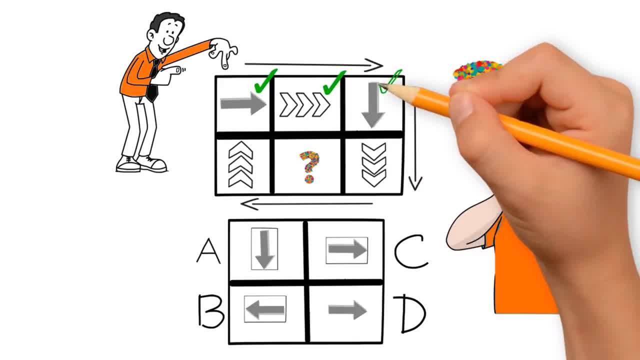 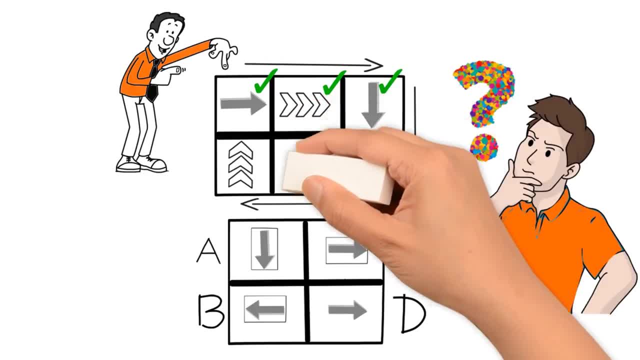 rotate clockwise. And then the third pattern, which is a little harder to identify, is that the previous arrow points to the next arrow's start. This is why the missing part, the part that you would need to identify, contains an arrow placed in the right corner pointing to the left. So the correct 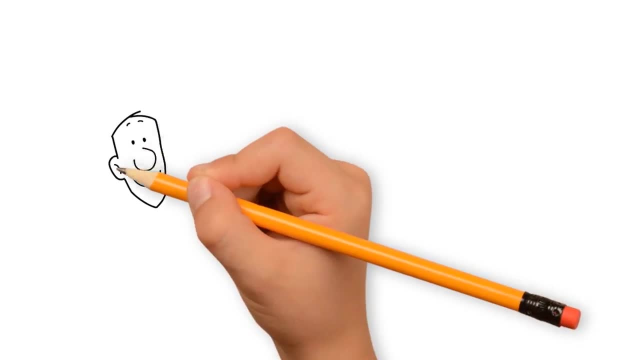 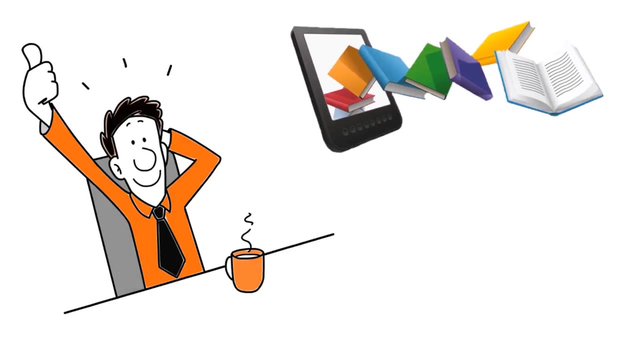 answer here is choice B. Hopefully you've nailed this question and now know how to answer similar problems in the test, But in case you need more problems and solutions, please make sure to check out my ebook in the description section of this video. 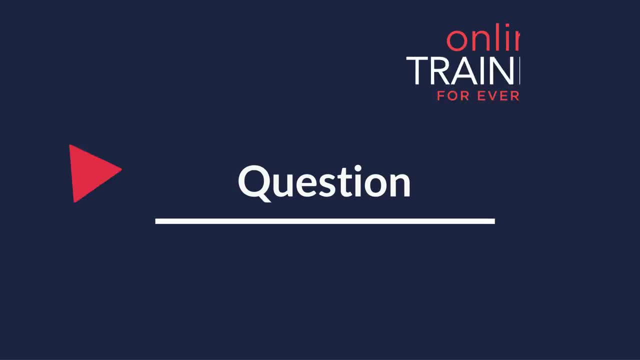 FACTORS OF THE 2X2 MAIN TEXT: 1. BUILDING A NUMBER OF TYPES OF QUESTIONS BY THE TOPIC DIFFERENCE B. 2. THE DIMENSION IN THE SYSTEM: 4 types of questions you are looking at is very frequently used on the test. Typically, you are: 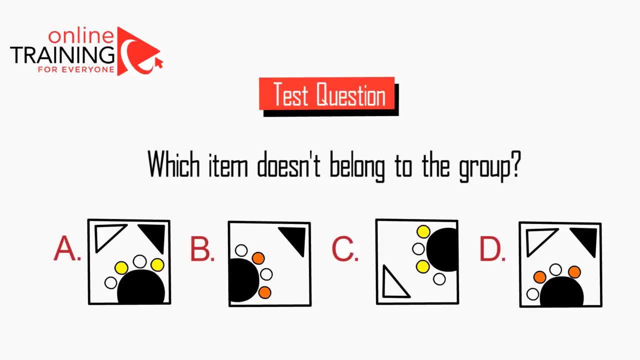 being asked to determine the item which does not belong to the group and you are presented with multiple items. In our choice, we have choices A, B, C and D. Each item is represented as a square which contains multiple different items inside and you need to determine the item which does not. 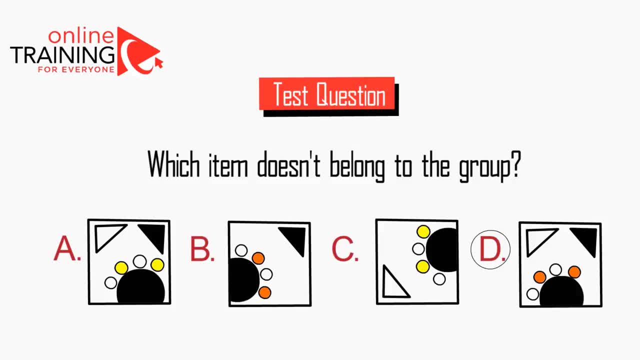 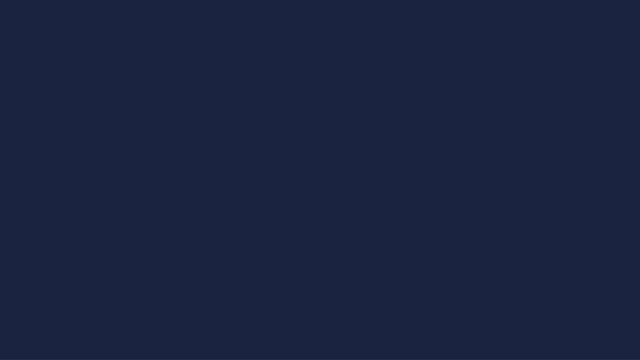 belong to this particular pattern or sequence. Do you see the answer? Please take a look to see if you can come up with the solution. Give yourself 5–10 seconds to see if you can come up with the answer. Did you figure it out? Let's continue to see how we can go and get to the correct solution. 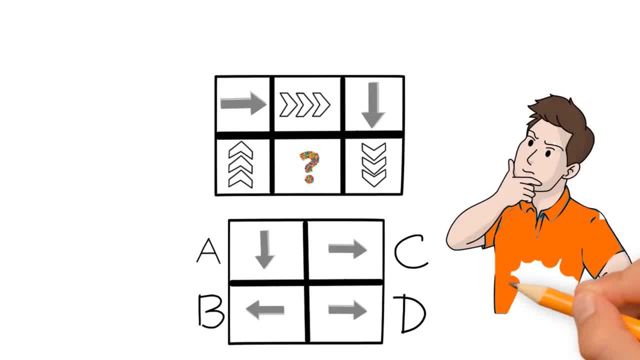 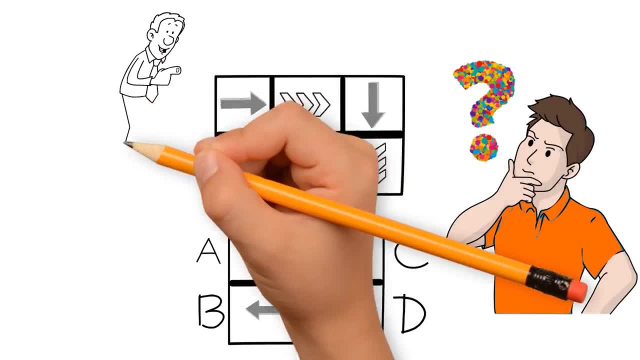 10 to 15 seconds to see if you can identify the right answer. Did you figure out the correct answer? Let's continue to see if we can get to the correct solution together. To solve these types of challenges, you always need to look for patterns. 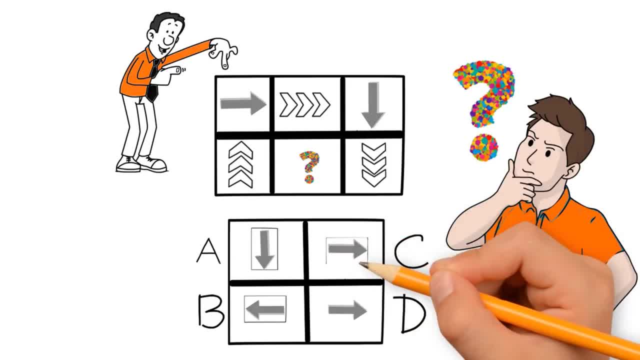 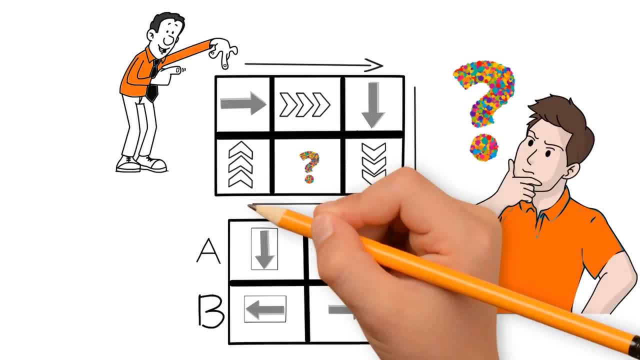 And there are three different patterns present in this sequence. Let's look at the pattern 1.. If we start from the upper left corner and go clockwise, you see that the arrows change alternatively in each subsequent box. Second pattern is that inside the box, solid arrows. 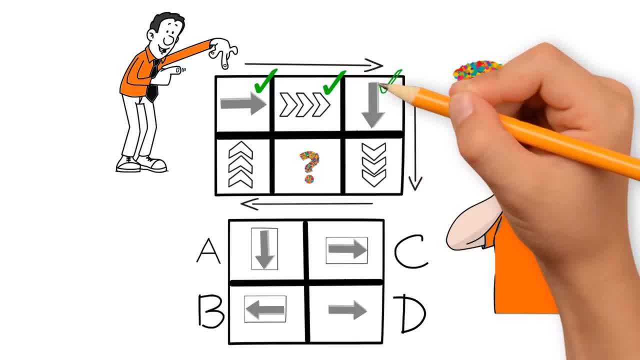 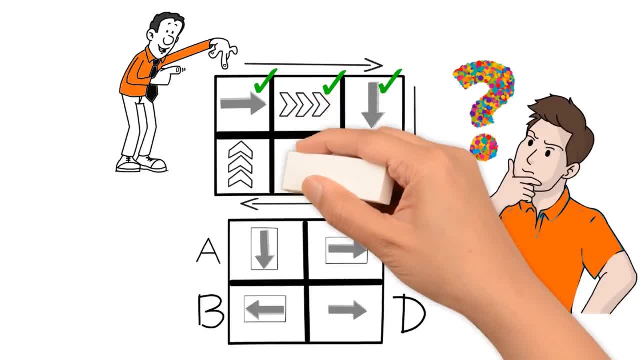 rotate clockwise. And then the third pattern, which is a little harder to identify, is that the previous arrow points to the next arrow: start. This is why the missing part, the part that you would need to identify, contains an arrow placed in the right corner, pointing to the left. 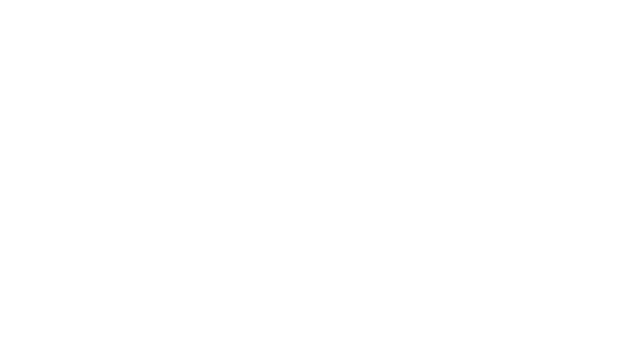 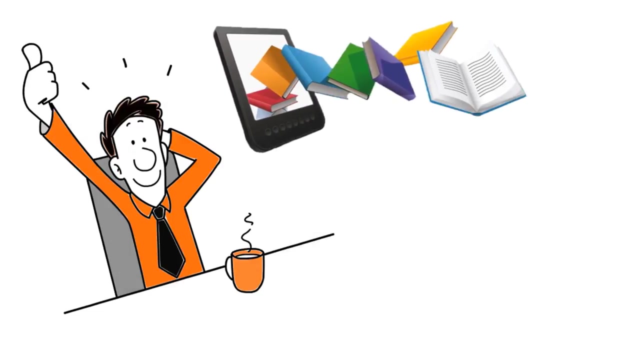 So the correct answer here is choice. Hopefully you've nailed this question and now know how to answer similar problems in the test, But in case you need more problems and solutions, please make sure to check out my ebook in the description section of this video. 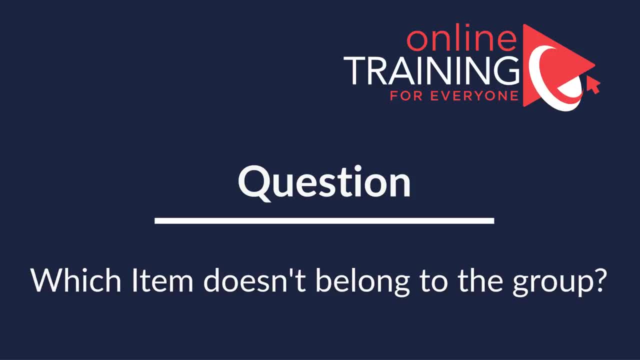 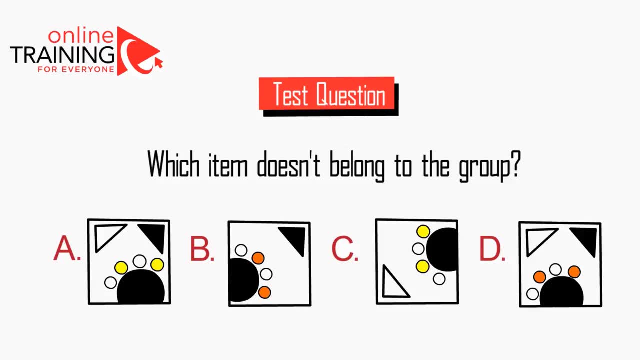 1917降浴 at is very frequently used on the test. typically, you're being asked to determine the item which does not belong to the group and you're presented with multiple items. in our choice, we have choices a, B, C and D. each item is represented as a square which contains multiple different items inside. 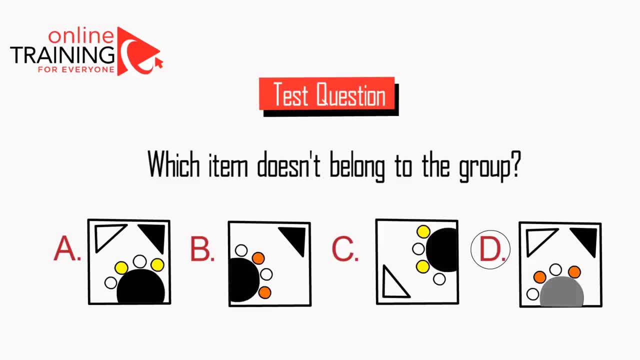 and you need to determine the item which does not belong to this particular pattern or sequence. do you see the answer? please take a look to see if you can come up with the solution. give yourself 5 to 10 seconds, maybe 10 to 20 seconds, to see if you can come up with the answer. did you figure it? 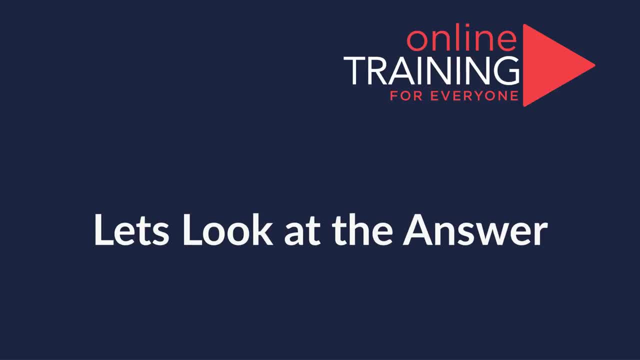 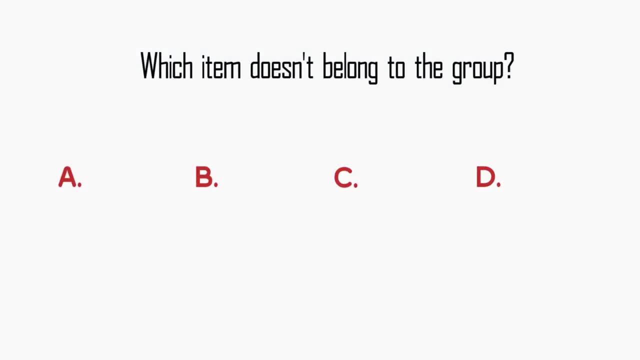 out. let's continue to see how we can go and get to the correct solution together. as you might have figured out by now, there is always a pattern that you need to detect to answer these types of questions correctly, and a lot of times there are items that are designed to confuse you. 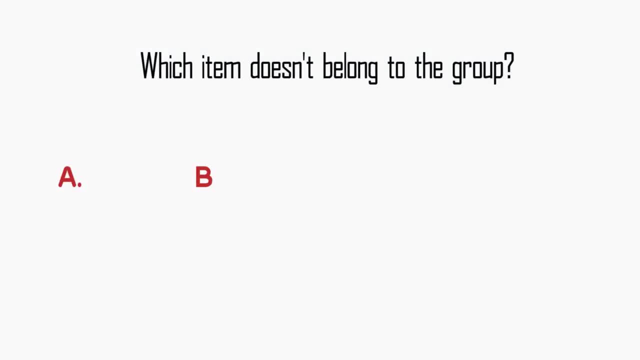 together. As you might have figured out by now, there is always a pattern that you need to detect to answer these types of questions correctly, and a lot of them are just in their own right to be answered. of times, there are items that are designed to confuse you, so let me first walk you through the 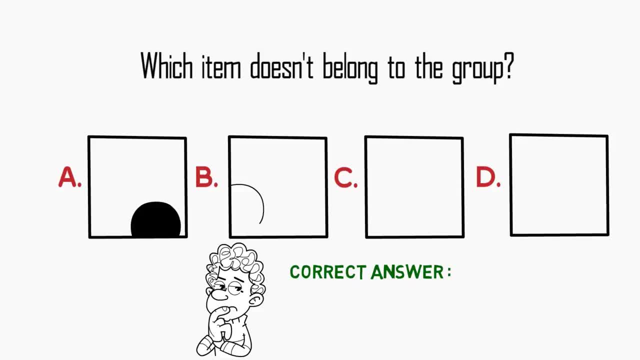 items that are designed to confuse you. you have small circles, and there are four small circles in each of the square, and the small circles do not have any patterns. we also have triangles. some squares have two triangles and some squares only have one, but there is no pattern here. the 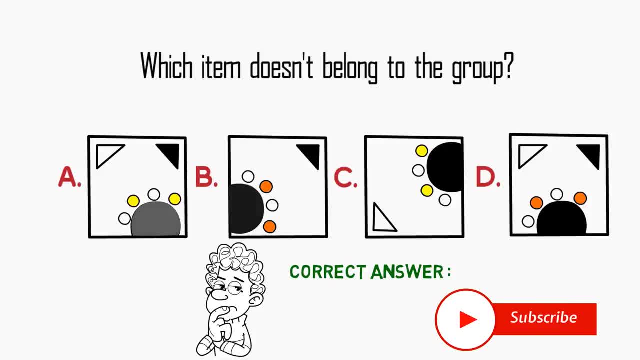 pattern is actually defined by the half circle and, as you can see, all half circles are attached to the corners of the square. you see this in the shapes a, b and c, but in shape d, half circle in placed in a different location. it is in the bottom middle of the square. this is why the item that 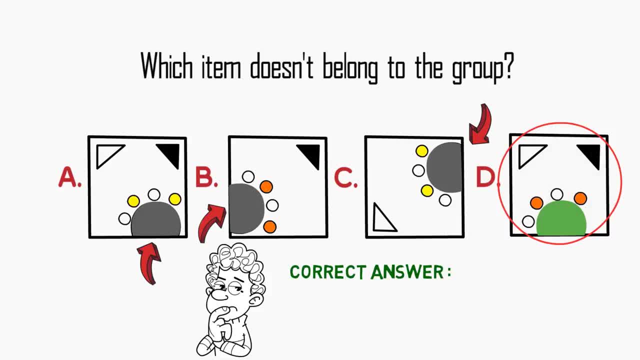 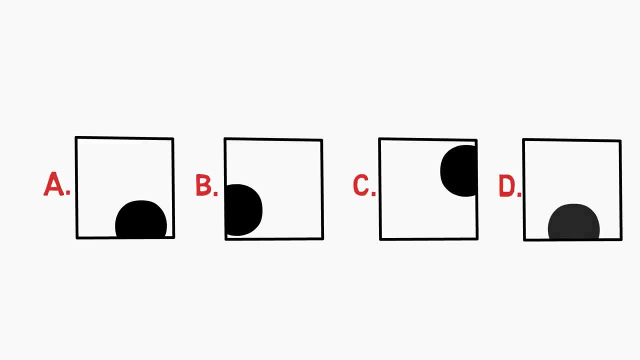 doesn't belong to the group is the choice d. so the correct answer here is choice d. let's recap: the pattern here is that all half circles are attached to the corners of the square, but half circle in the shape d is placed in a different place than the others. the half circle there is in the lower part. 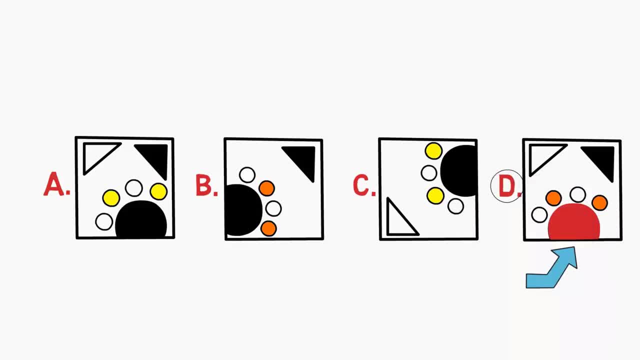 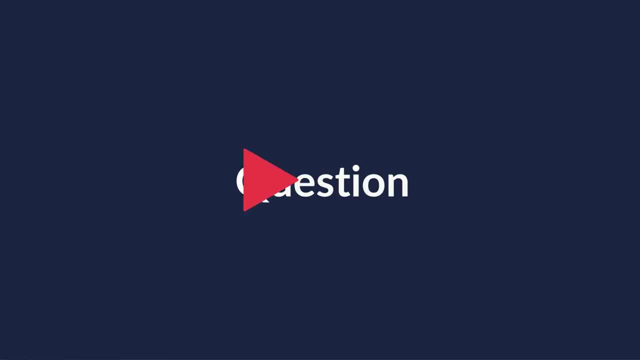 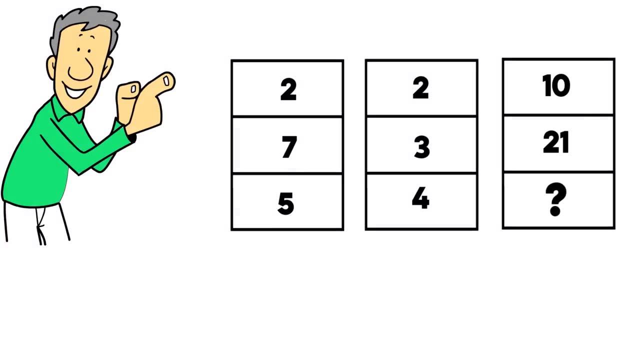 of the square. this is why the correct answer here is choice d. hopefully you've nailed this question and now know how to answer similar problems on the test. i'm extremely excited to share with you the question that tests your pattern recognition skills. you're presented with three columns. 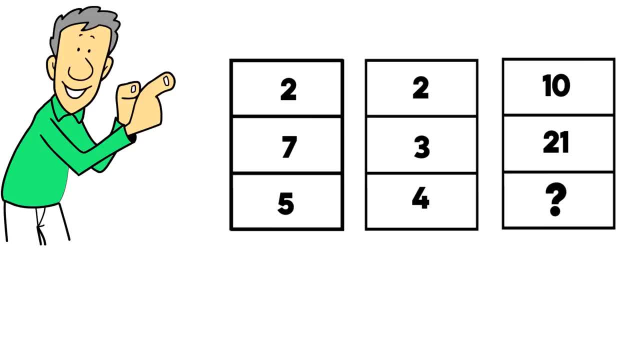 each column has three numbers. in the first column we see numbers two, seven, five. in the second middle column, we see numbers two, three and four, and in the last rightmost column, column number three, we see numbers 10, 21 and then one number missing. you need to find the missing value which is highlighted. 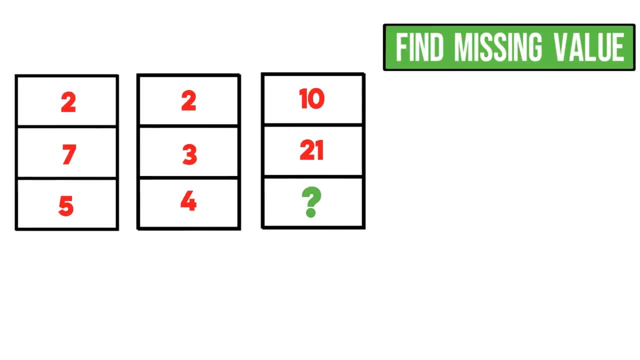 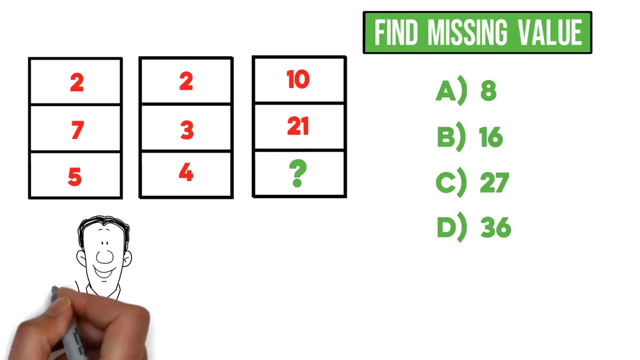 by question mark. you need to find the missing value and you have four choices to choose from: choice a- 8, choice b- 16, choice c- 27 and choice d- 36. do you think you can recognize missing value? give yourself five to ten seconds to see if you can come up with the answer. 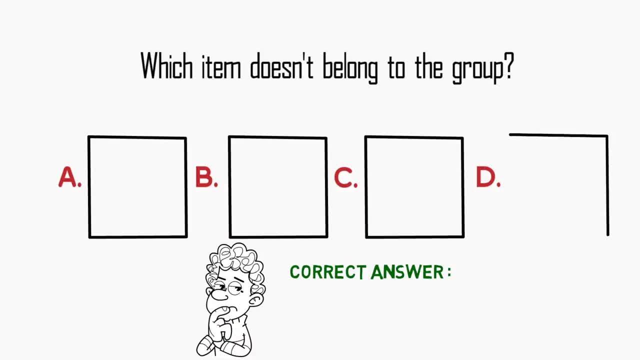 so let me first walk you through the items that are designed to confuse you. you have small circles, and there are four small circles in each of the square, and the small circles do not have any patterns. we also have triangles. some squares have two triangles and some squares only have one, but 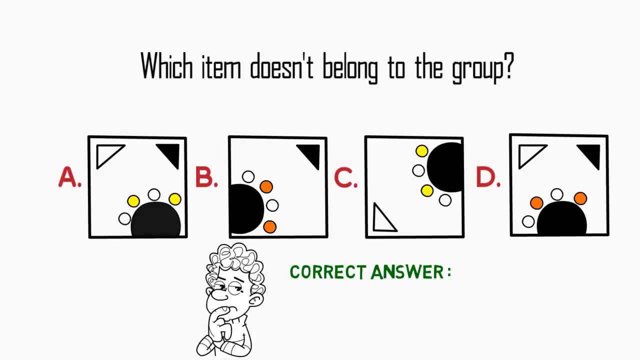 there is no pattern here. the pattern is actually defined by the half circle and, as you can see, all half circles are attached to the corners of the square. you see this in the shapes A, B and C, but in shape D, half circle in placed in a different location it. 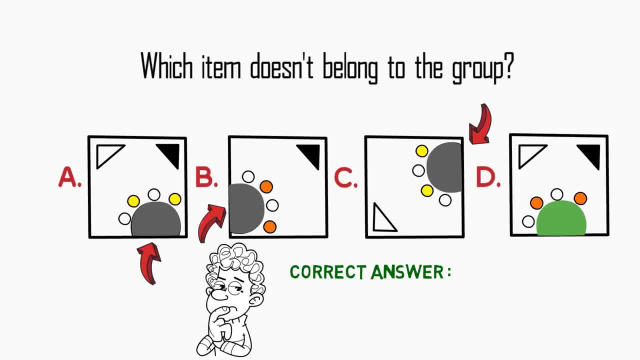 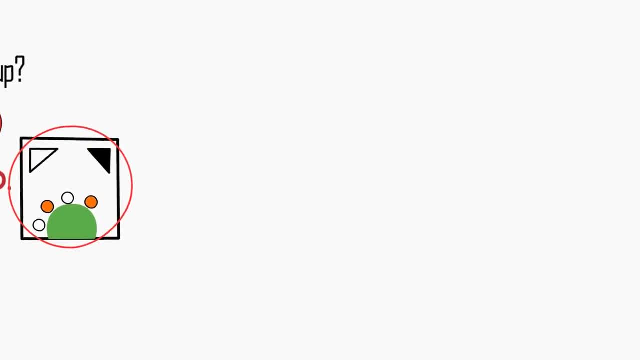 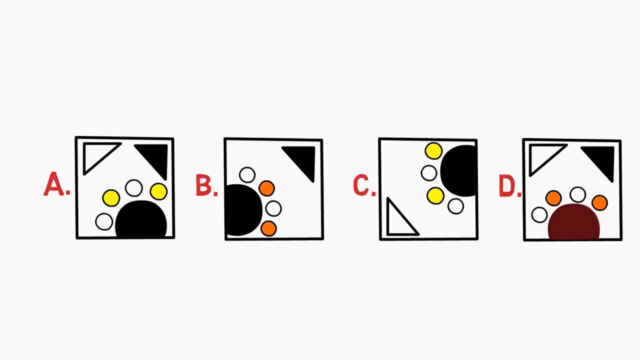 is in the bottom middle of the square. this is why the item that doesn't belong to the group is the choice D. so the correct answer here is choice D. let's recap: the pattern here is that all half circles are attached to the corners of the square, but half circle in the shape D is placed in a. 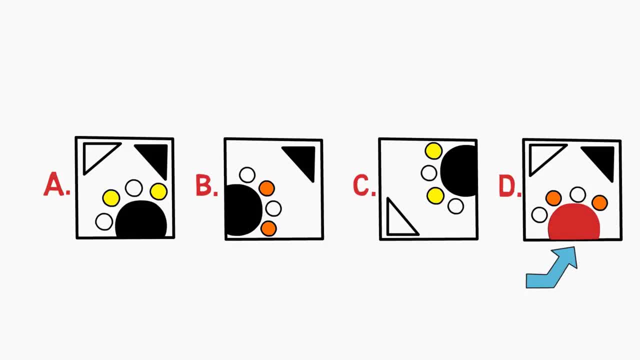 place than the others. the half circle there is in the lower part of the square. this is why the correct answer here is choice D. hopefully you've nailed this question and now know how to answer similar problems on the test. I'm extremely excited to share with you the question that 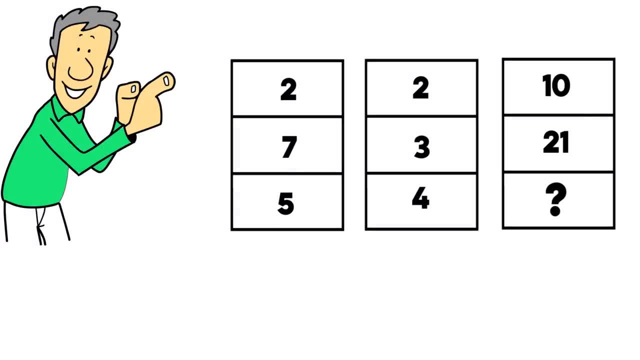 tests your pattern recognition skills. you're presented with three columns. each column has three numbers. in the first column we see numbers two, seven, five. in the second middle column, we see numbers two, three and four. and in the last rightmost column, column number three, we see numbers 10, 21 and then one number missing. you need to find the missing value, which is highlighted by 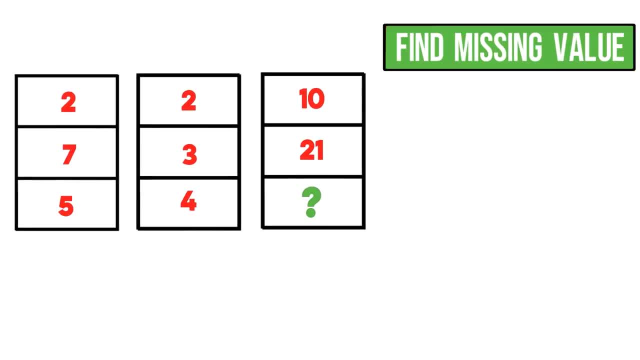 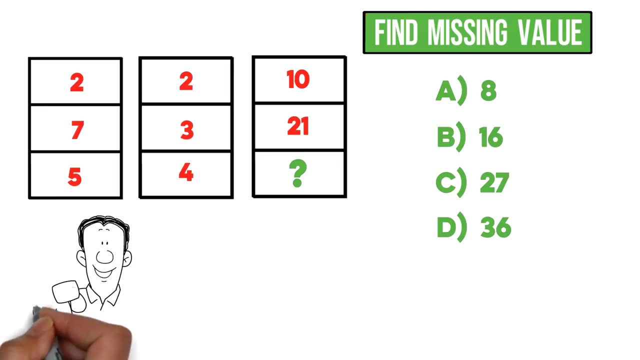 question mark. you need to find the missing value and you have four choices to choose from: choice A- 8, choice B- 16, choice C- 27 and choice D- 36. do you think you can recognize missing value? give yourself five to ten seconds to see if you. 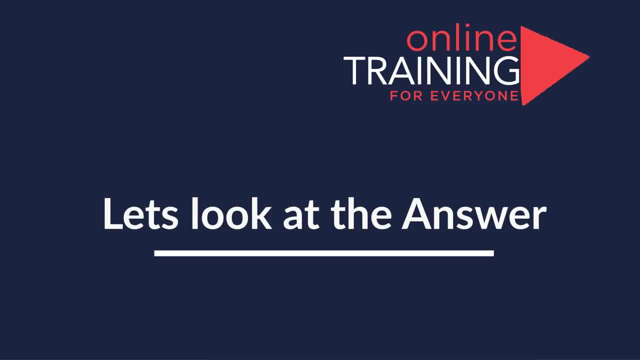 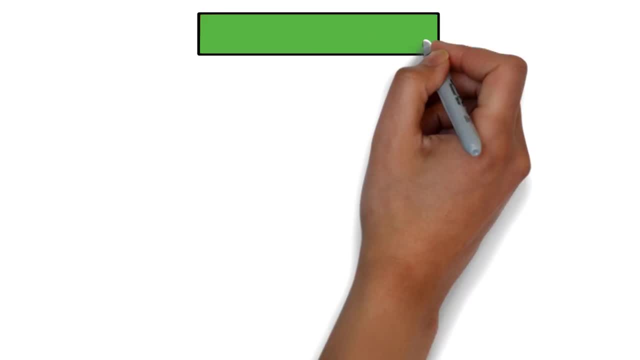 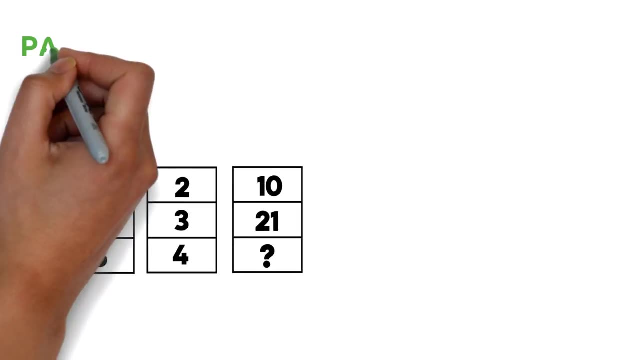 can come up with the answer. did you figure out the solution? let's continue to see how we can get to the correct solution together. the most important skill to solve these types of problems is pattern recognition skill. to recognize the pattern you need to look closely into each column. selective values in columns one and two by multiplication: 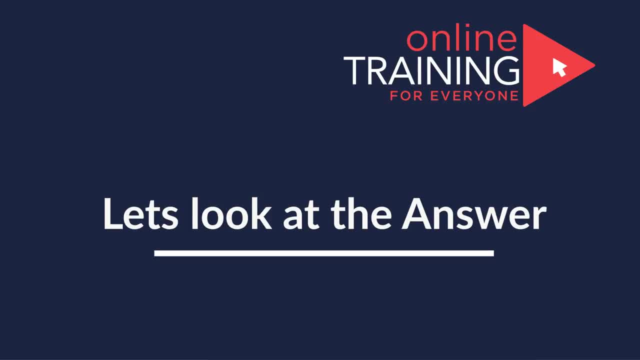 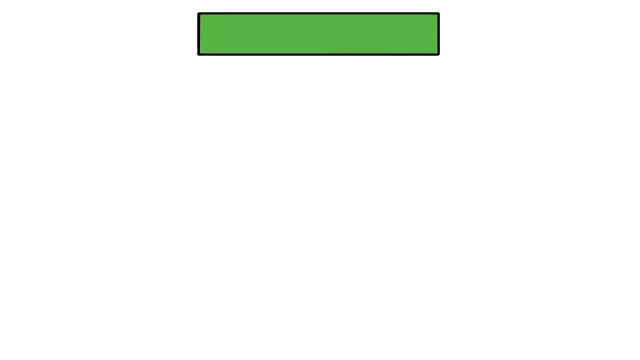 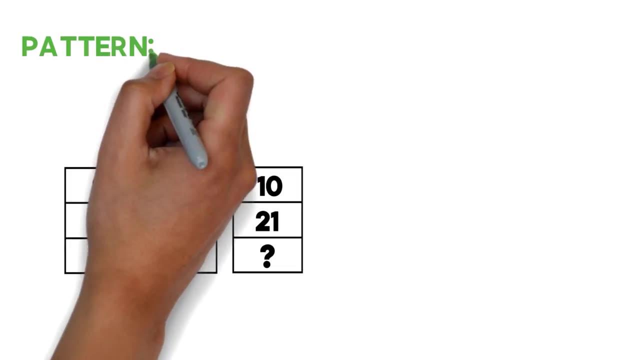 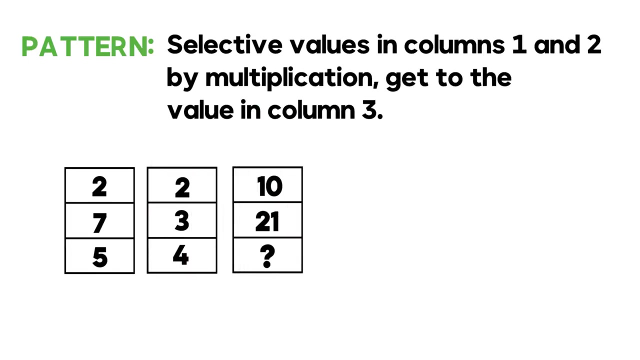 did you figure out the solution? let's continue to see how we can get to the correct solution together. the most important skill to solve these types of problems is pattern recognition skill. to recognize the pattern you need to look closely into each column. selective values in columns 1 and 2: by multiplication, get to the value in column 3. 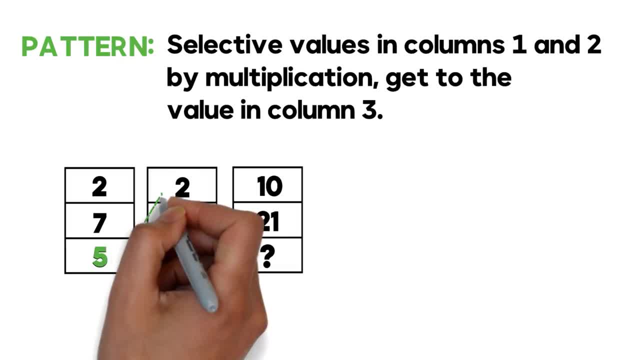 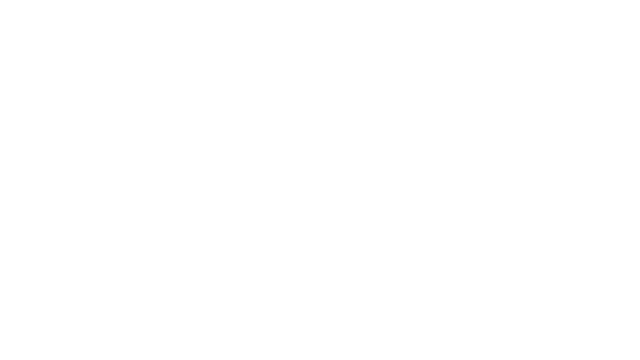 and this is our pattern. let's take a closer look for the values that already present. if we multiply 5 by 2, we get to the value of 10.. second set of values represented by the middle row, 7, multiplied by 3, equals 21.. so the second set of values represented by the middle row, 7, multiplied by 3, equals 21.. 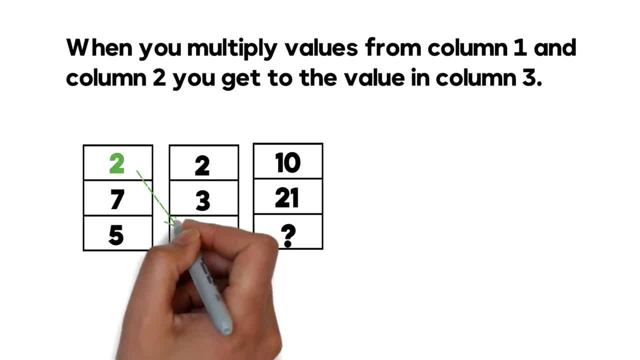 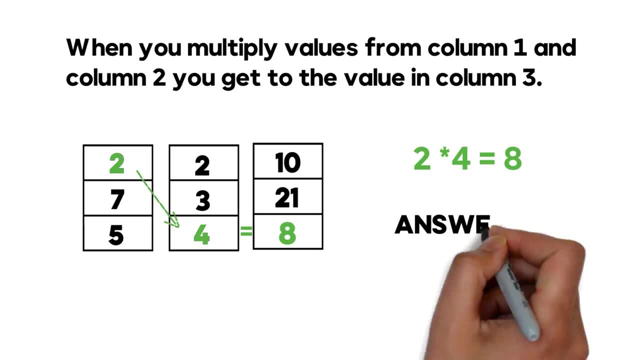 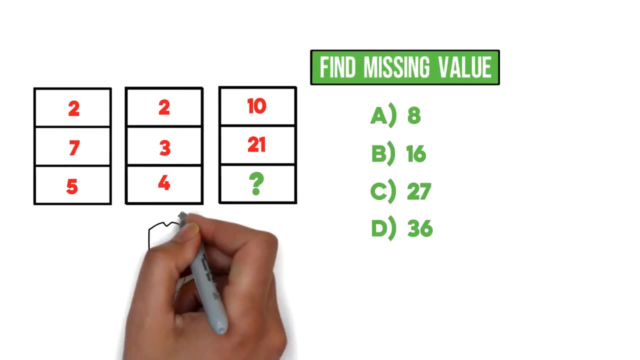 the missing values here can be calculated by multiplying 2 by 4, and the end result would be equal to 8.. so the correct answer to this problem is choice a 8.. i also wanted to share with you one of the typical mistakes people make as part of answering these types of questions. 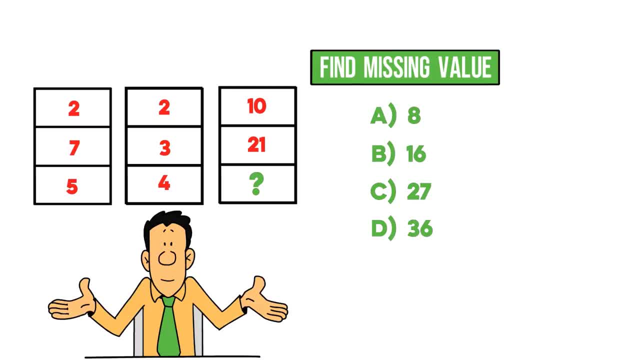 people start looking at the columns themselves, but unfortunately there's no pattern just by looking in the values in column one, since pattern just doesn't exist If you look only at the values in column 1, or only at the values in column 2, or only 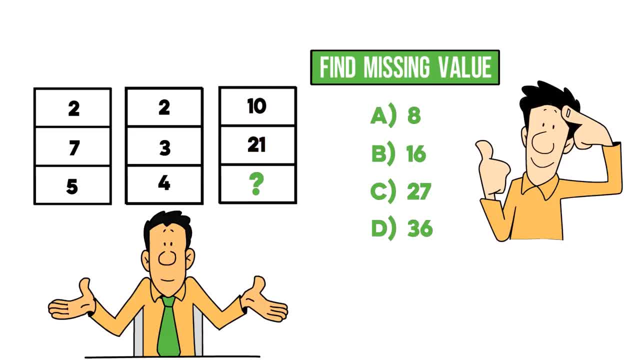 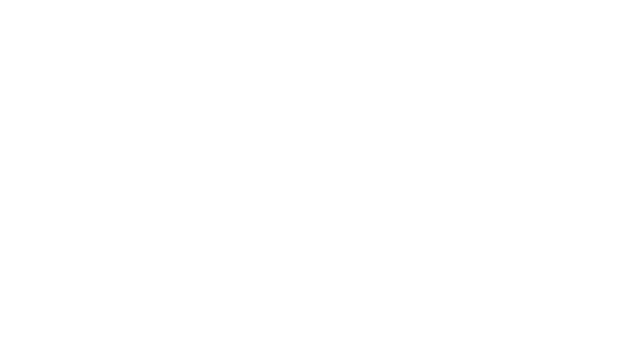 at the values in column 3, you will not be able to come up with the answer. You have to look across and take a global view across multiple columns to get to the correct solution. Can you do me a favor? If you have a better way of solving this challenge, please share your thought process in the comment. 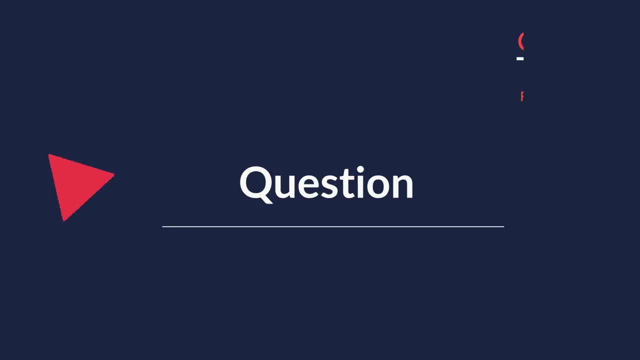 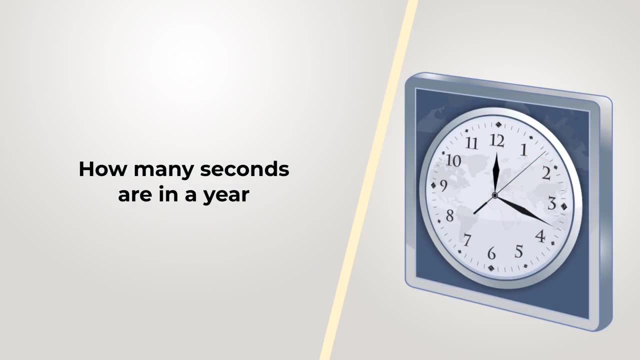 section of this video. I had this question being asked as part of consulting job interview: How many seconds are there in a year? Take a look at the picture. It might give you a hint. Do you think you know the answer? Think of the logic. how would you calculate how many seconds are there in a year? 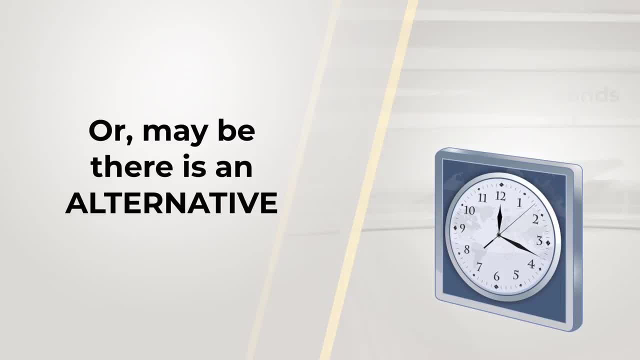 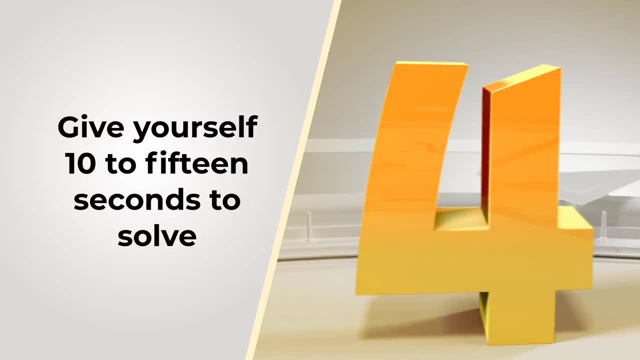 Or maybe there is an alternative. Always try to think out of the box- This would be my hint to you- And give yourself 10 to 15 seconds. This is as much time as you might get answering these types of questions in a time. 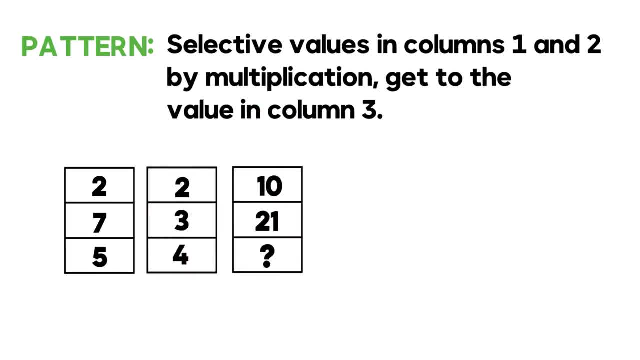 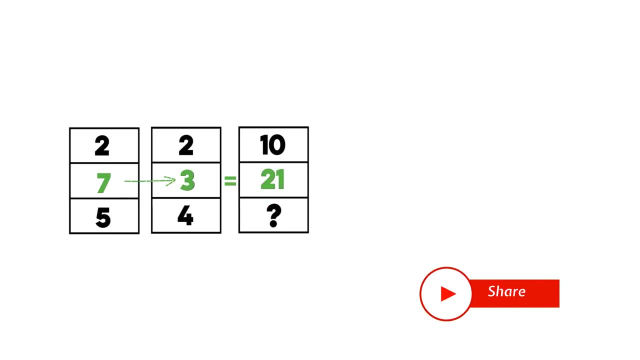 get to the value in column three, and this is our pattern. let's take a closer look for the values that already present. if we multiply 5 by 2, we get to the value of 10.. second set of values, represented by the middle row: 7 multiplied by 3 equals 21.. so the missing values here can be: 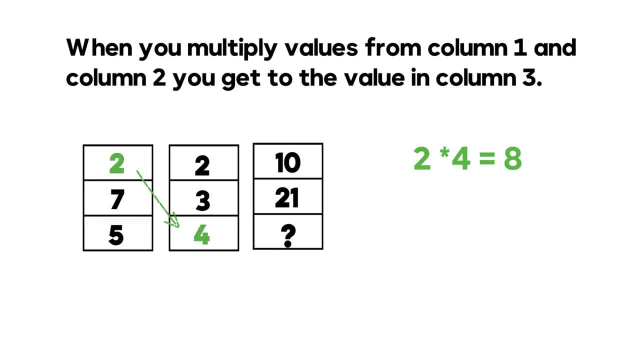 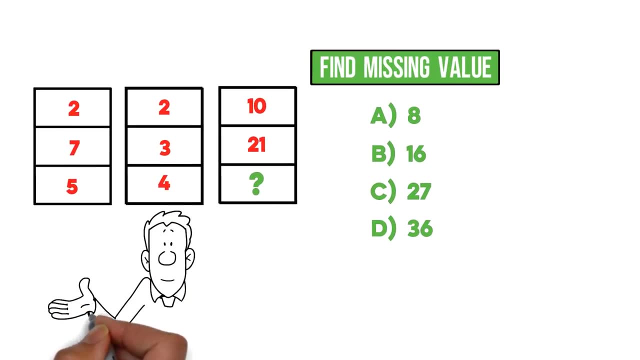 calculated by multiplying 2 by 4, and the end result would be equal to 8.. so the correct answer to this problem is choice A 8.. I also wanted to share with you one of the typical mistakes people make as part of answering these types of questions: people start looking at the columns themselves. 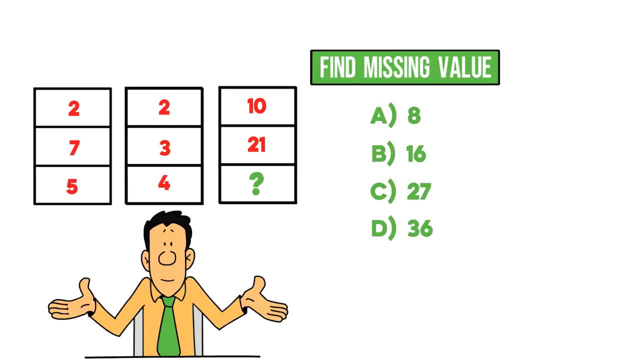 but unfortunately there's no pattern just by looking in the values in column one, since pattern just doesn't exist. if you look only at the values in column one or only at the values in column two or only at the values in column three, you will not be able to come up with the answer. 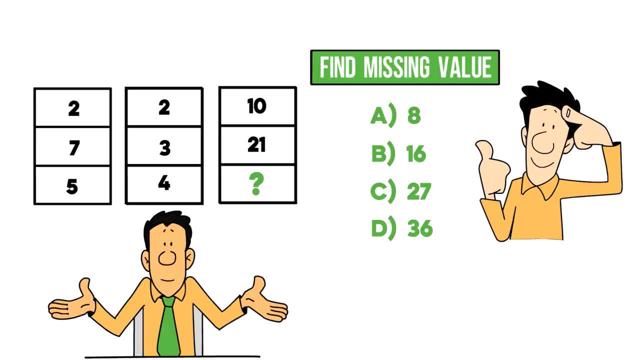 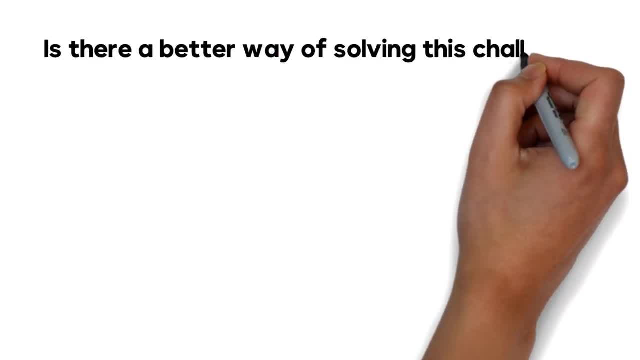 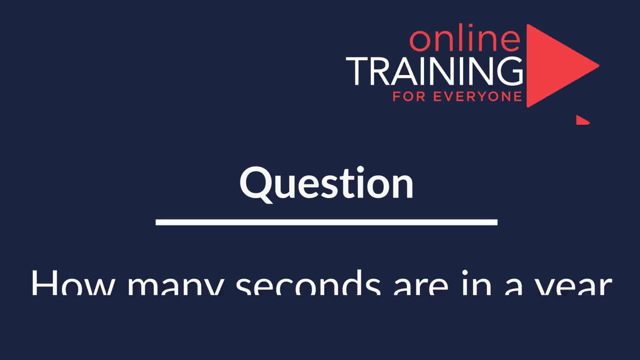 you have to look across and take a global view across multiple columns to get to the correct solution. can you do me a favor? if you have a better way of solving this challenge, please share your thought process in the comment section of this video. I had this question being asked as. 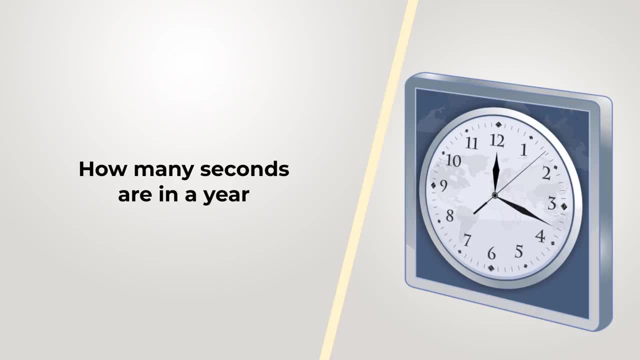 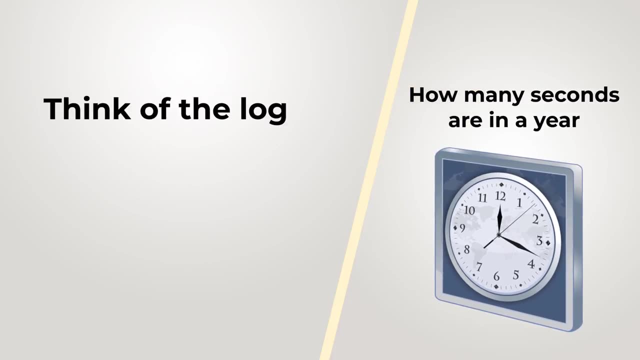 part of consulting job interview. how many seconds are there in a year? take a look at the picture. it might give you a hint. do you think you know the answer? think of the logic. how would you calculate how many seconds are there in the year? or maybe there is an alternative. always try to think out of the 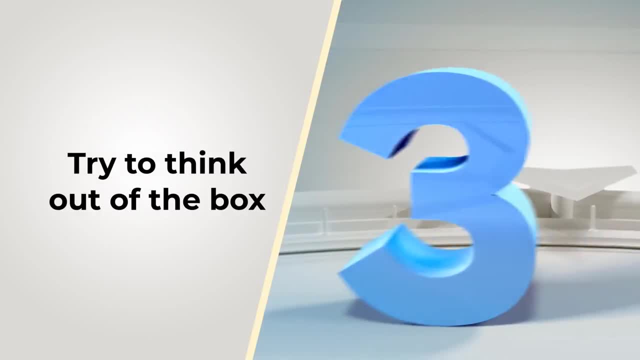 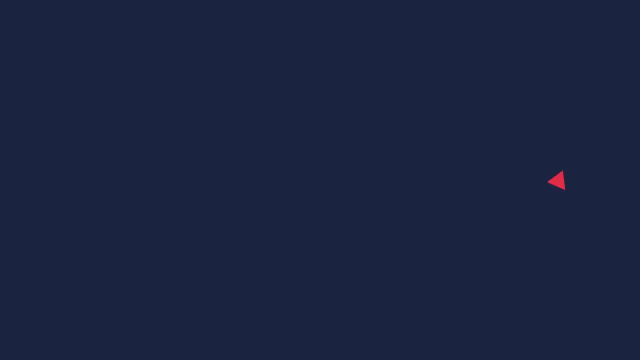 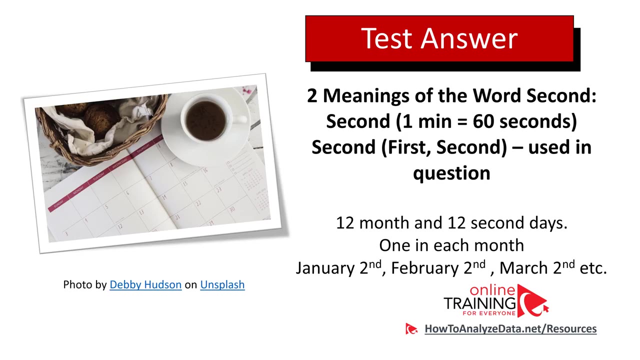 box- this would be my hint to you- and give yourself 10 to 15 seconds. this is as much time as you might get answering these types of questions in the test. now let's continue and get to the correct solution together. obviously, this is a tricky question. 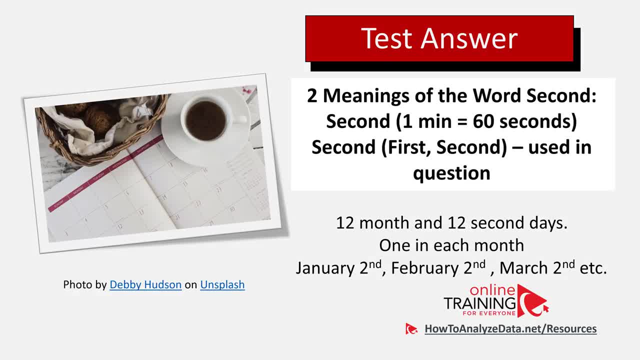 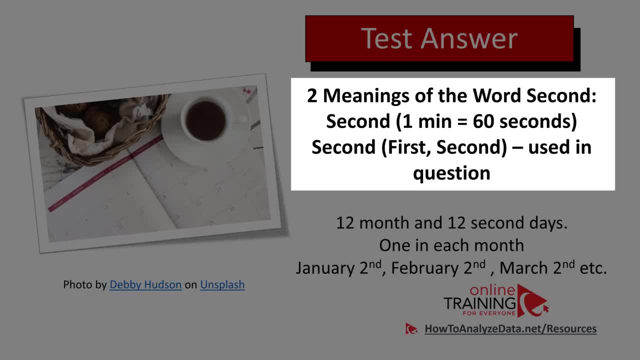 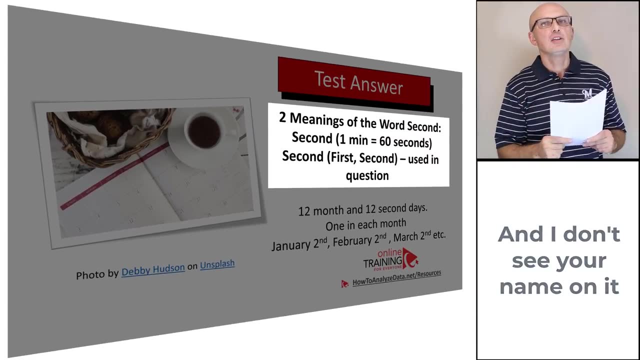 and it challenges you in understanding of the word second. there are two meanings in the word second. one is second- for example, one minute has 60 seconds- but second one is second, where you have sequence of first and second and the second meaning of the second is used in this particular question.